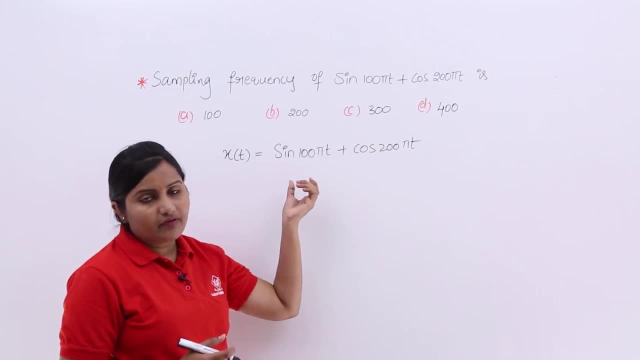 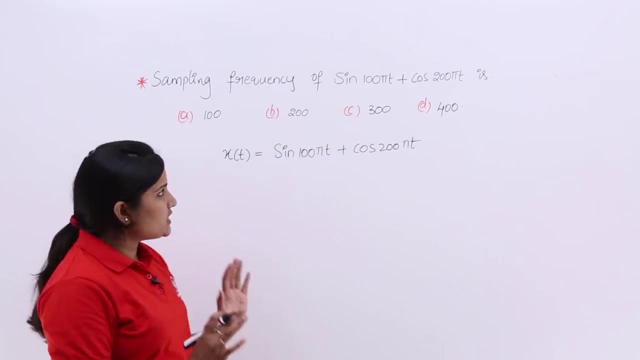 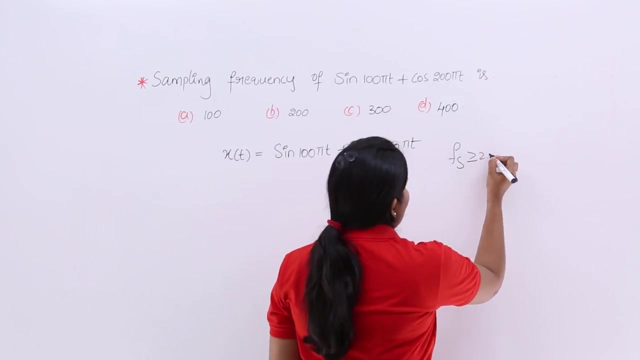 component means. So here we need to find out the individual frequency components and maximum of that will work as a frequency component of message signal. So generally, what they are asking is sampling frequency. you know that. So sampling frequency must be greater than or equivalent to 2 fm. The minimum sampling frequency is. fs is equivalent to at least. 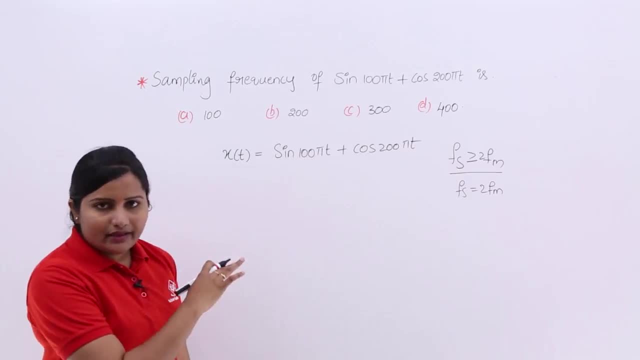 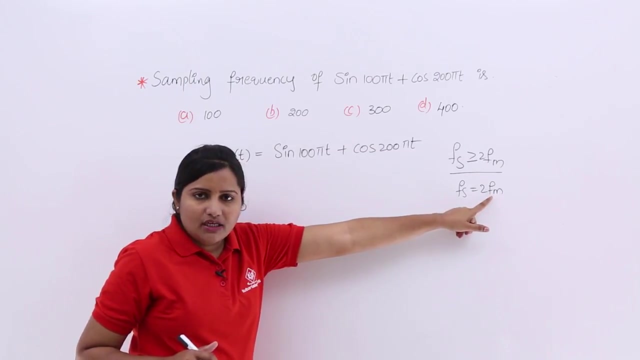 equivalent to 2 fm. you need to consider So greater than 2 fm. any value is advisable to get perfect sampled signal and to recover your message signal again. So here to get fs you need 2 fm. that means fm value, but you are not given with any fm value here. 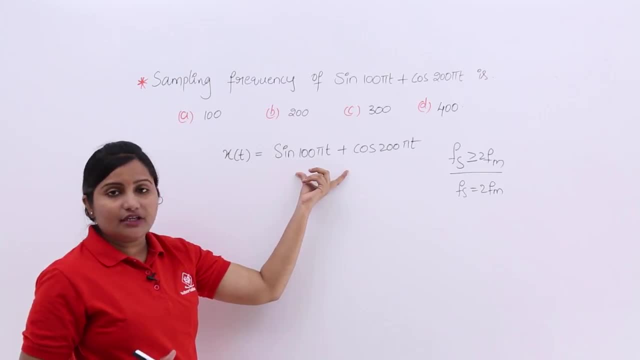 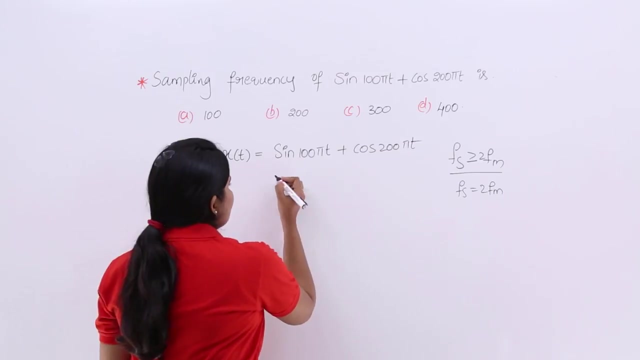 They just given signal. So you are given signal directly from this signal you need to calculate fm. How you can get fm means here you are having 2 frequency component. In that 2 frequency component, which component will be message component that we need to see? So here I am considering a calculation. 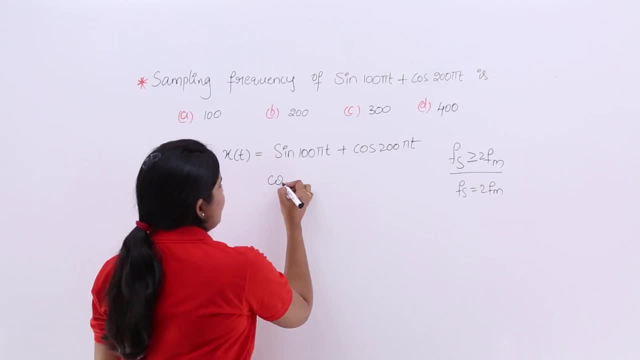 of first frequency component. I am just comparing with sin omega t. So omega 1 is equivalent to 100 pi, So 2 pi f is equivalent to 2 pi. f. 1 is equivalent to 100 pi, So this is equivalent to 50 times. So f 1 is equivalent to 50 heads. The first frequency. 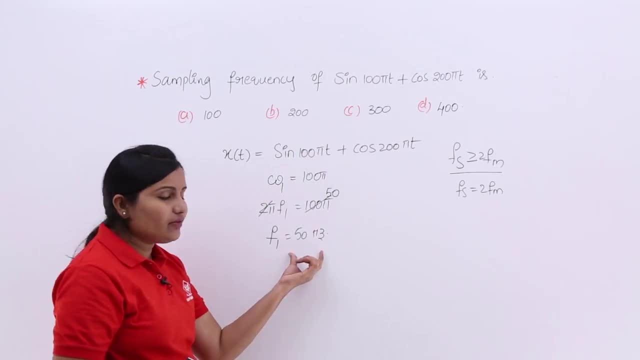 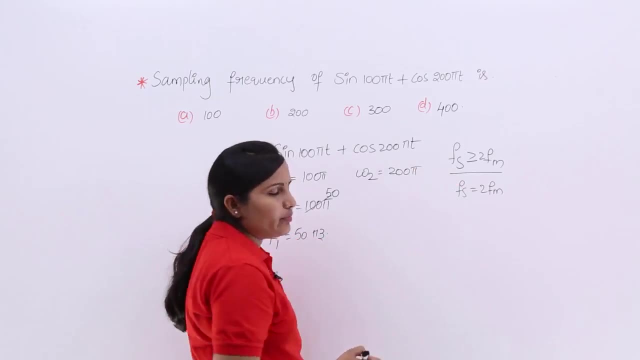 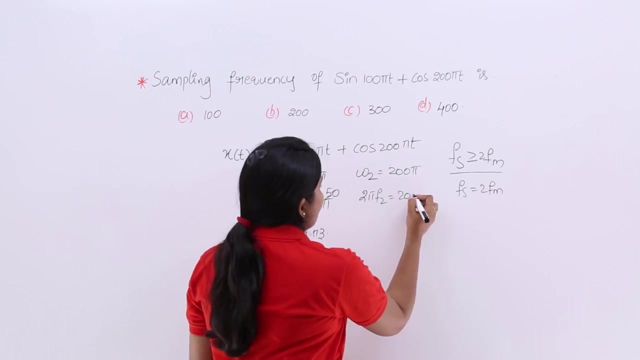 component in this signal, in the message signal, is equivalent to 50 heads. Now coming to 2nd frequency component, that can be calculated like this. I am considering like omega 2, I am just comparing with cos, omega t, So 2. pi f: 2 is equivalent to 200 pi, So here 2. 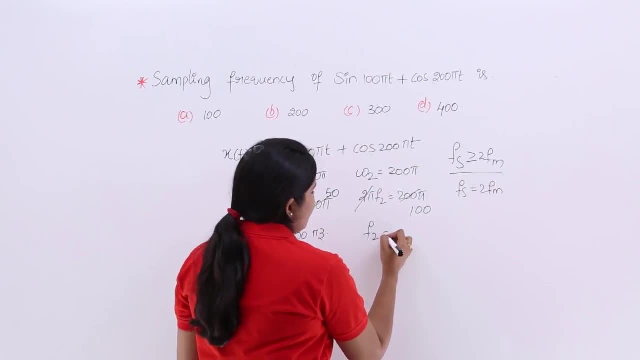 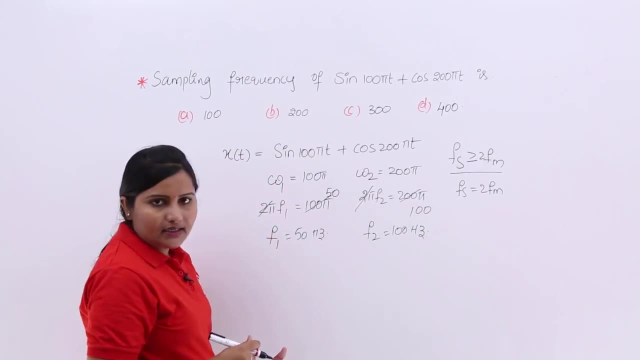 pi hundred times will go. So this will be equal to 50 heads. So I can calculate like. So f 2 is equivalent to 100 heads. Now you can calculate f m. the message frequency component is the maximum frequency component in the combination of frequency components in the 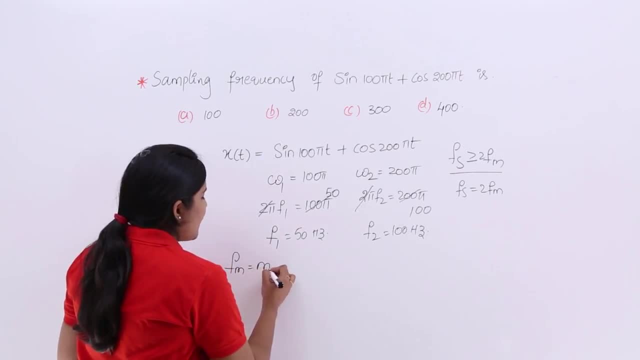 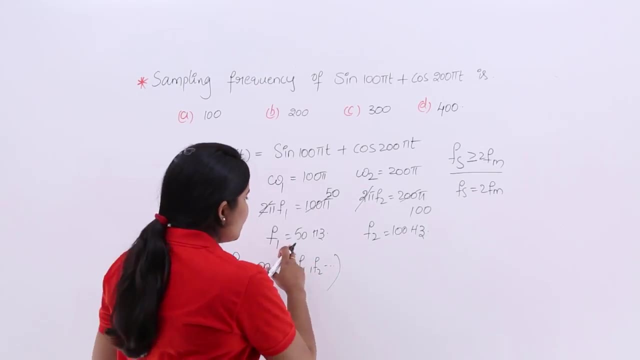 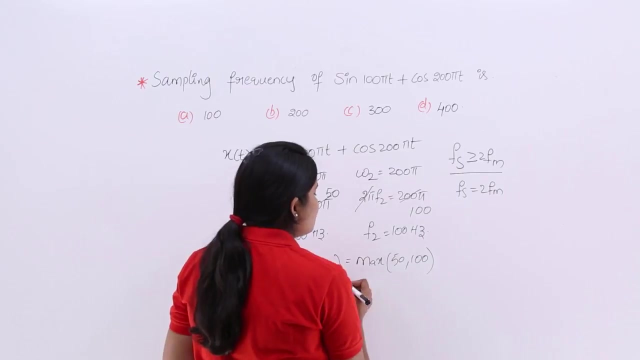 message. So that means f m is equivalent to you are having a formula maximum of f 1 comma, f 2 comma, so on, For example if you are having more components. So here you are having 2 components And so maximum of 50 comma. 100 means in 50 heads and 100 heads. the maximum frequency is 100 heads. 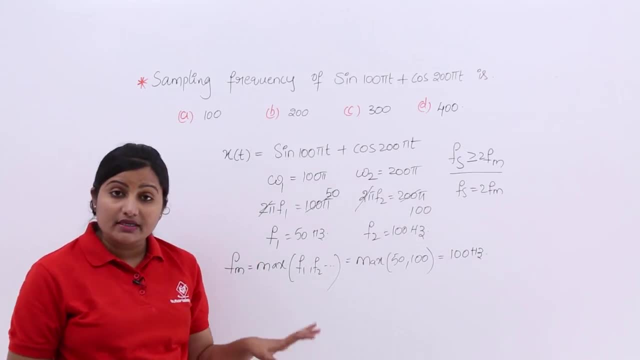 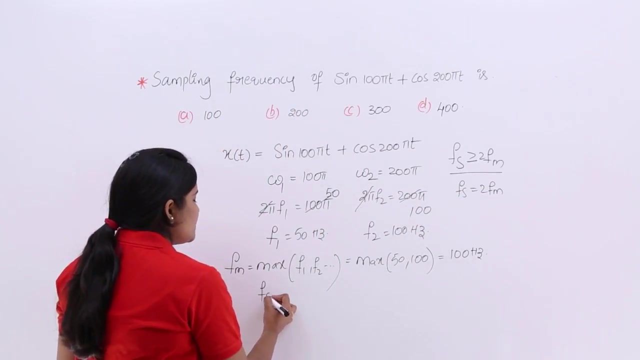 This will become the frequency component of message: message frequency. This can be considered as message frequency. Now you are having your message frequency in your hand, Then this is the time to calculate sampling frequency. So I am substituting in that f s. 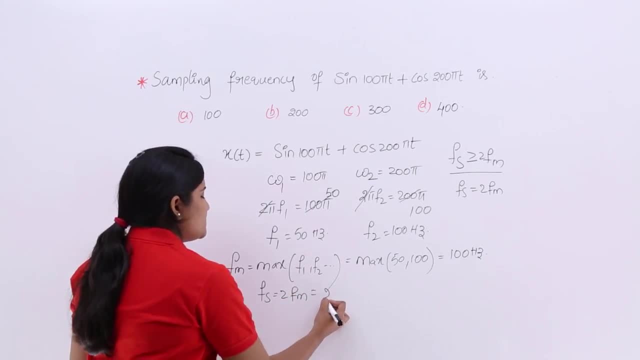 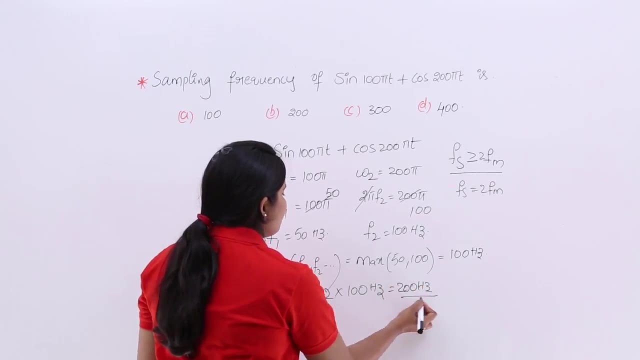 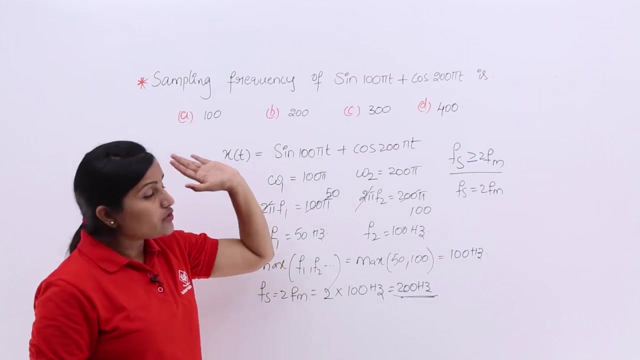 is equivalent to 2 f m. So if f s is equivalent to 2 f- So I am multiplying with this 100 H- then you are going to get 200 H as your Fs. you can see So in the options. they given 200, 300, 400, like this. So whenever they are. 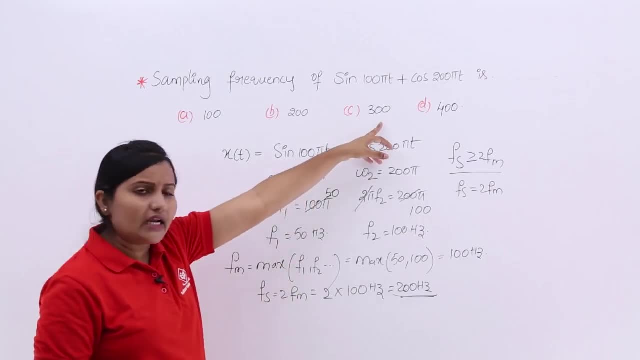 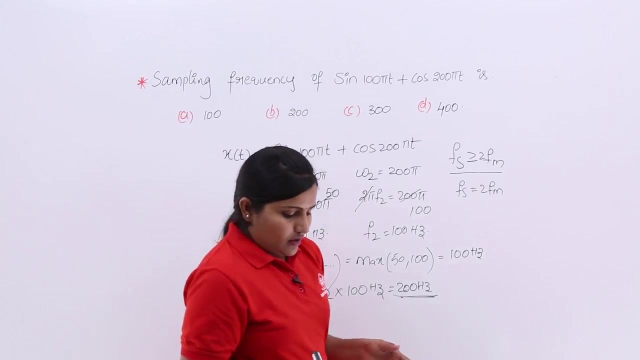 giving just what is the sampling frequency? you can take 300 also. you can take 400 also. When this type of problems are given in technical exams, you need to consider options like Nyquist frequency. that is it So in in in previous days. they are not used to give like this. that. 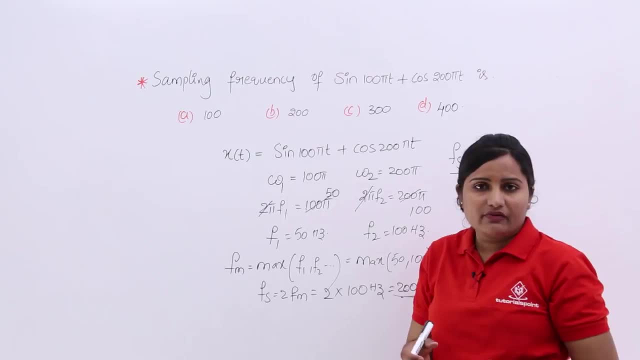 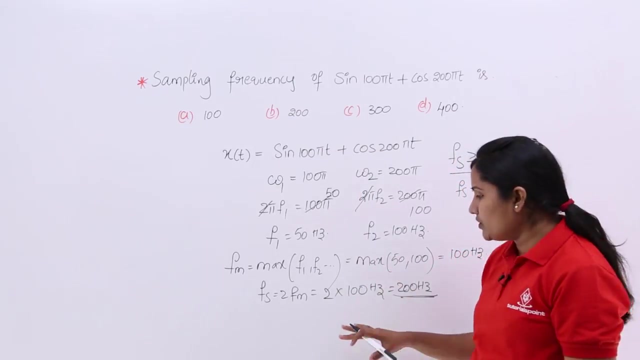 means they are specifying what is the minimum sampling frequency or what is the minimum sampling prime frequency or what may be. the Nyquist state like that they are asking. For example, if they are not asking like that, they are just asking sampling frequency also, you can take minimum sampling frequency. 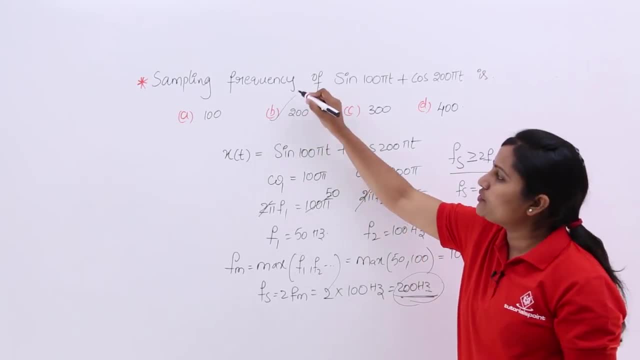 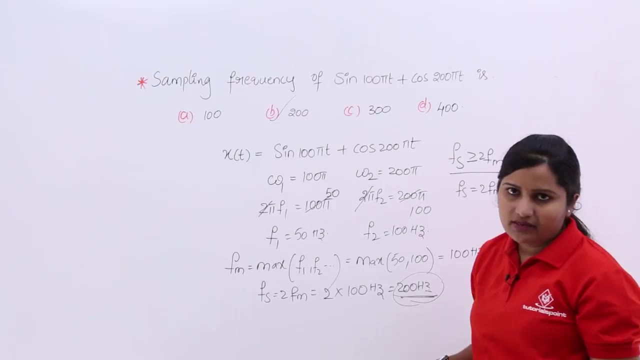 So this 200.. 200 H Nyquist rate you need to consider to sample this signal, this message signal, to sample this message signal without any distortion, the signal frequency, sampling prime frequency that you need to consider, that must be 200 H at least. So at most that may be anything. 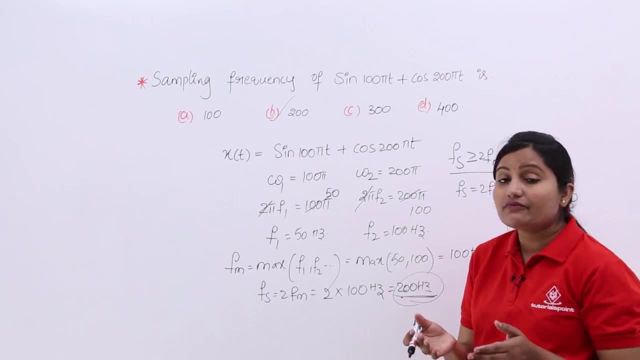 you can take so much. that means Fs, for example. if you consider so much greater than 2 Fm, what will happens? So the data rate is going to waste. that means so if you are using more than enough, then definitely your data bits are going to exceed. you are going to your. your data is converting. 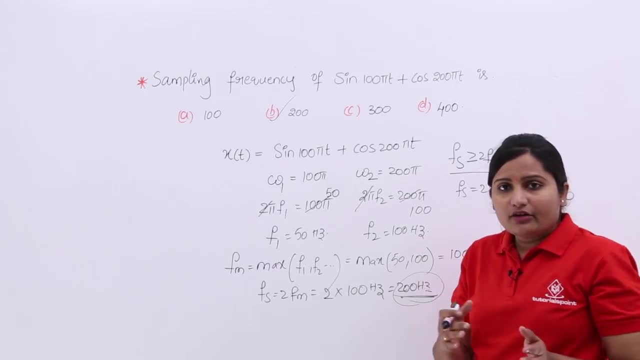 into more number of bits. it will take more data rate to transfer more number of bits. it will take more cost to transfer more number of bits. So our wish is to transfer our message. for that, whatever required up to that, we will take more than that not required. if you consider more than that, you can transfer perfectly.